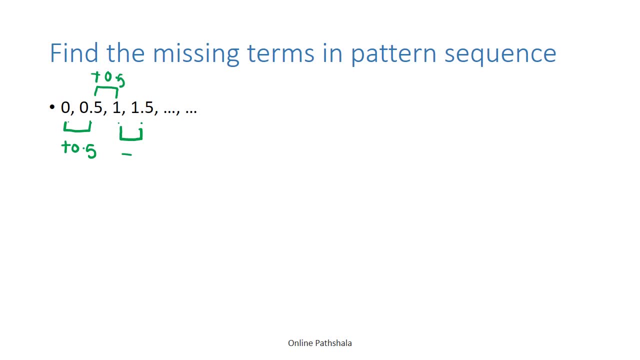 Same way: 1 to 1.5, the increment is of 0.5.. So the next term will again have an increment of 0.5.. 1.5 plus 0.5. Will give us 2.. 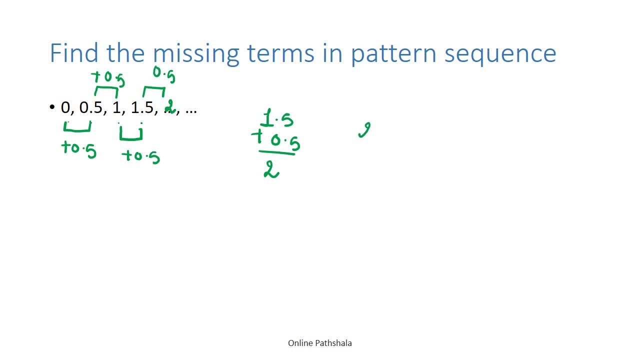 So the next term will become 2.. And 2 plus 0.5 will give us 2.5.. So the next term after 2 will be 2.5.. So the steps are: first you find out the increment. 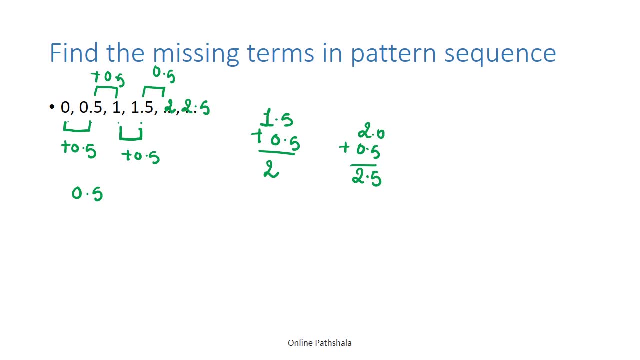 To find out the increment, take up the bigger number, Subtract the smaller previous number from it, You will get the increment, and then you have to add the increment to the next number which you are going to find out to find out the next number. 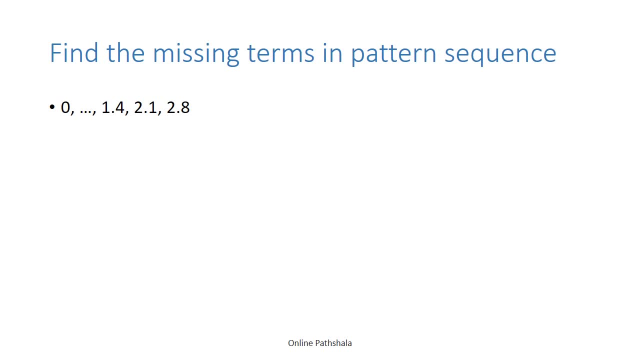 Let us look at one more example where we have to find out a left hand side number. So here again, the first step is to find out the increment. The increment between 2.8 and 2.1 is of 0.7.. 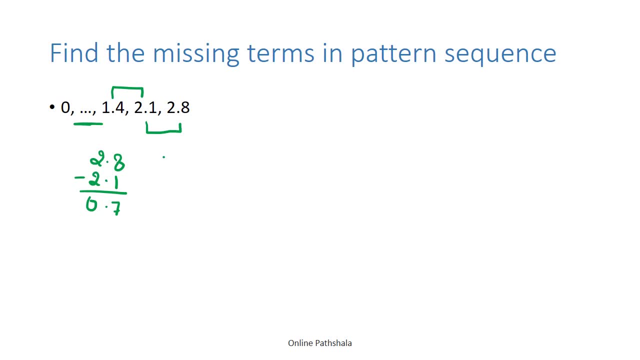 Same way, the increment between 1.5.. 2.4 and 2.1 is 2.1 minus minus 1.4. That is again 0.7.. So it is clear after checking for the two numbers that the increment is of 0.7.. 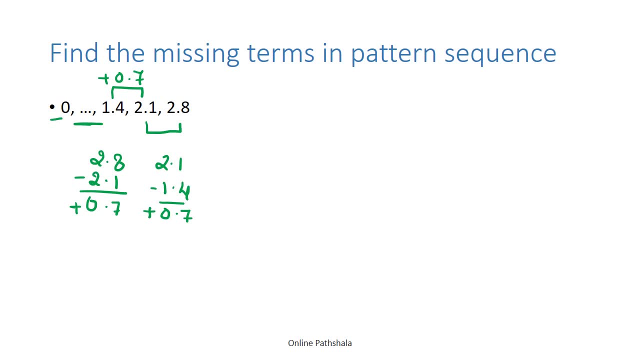 So there are two ways of doing it: Either as this blank is on the right hand side, or is more bigger than 0.7.. We can add 0 and 0.7.. That gives us 0.7 as our number. 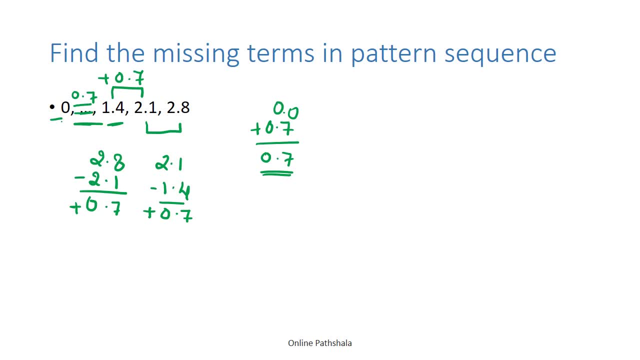 Or another way is, as it is, on the left hand side of 1.4.. 1.4, left hand side, Left hand side. So we can subtract from 1.4. So as to get us 0.7..